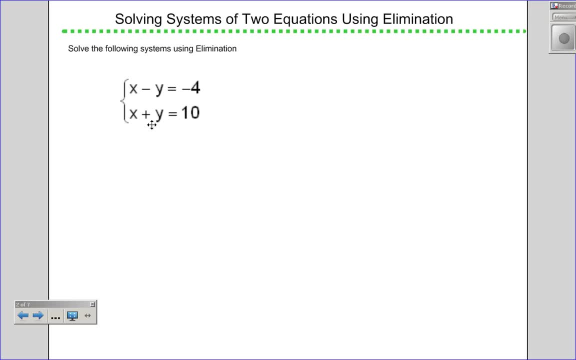 So there's- really- I need to start thinking about this in a different way- And I do notice that I have one variable, this minus y, and a positive y, and they're opposites. So what I can do is combine them, my two equations. 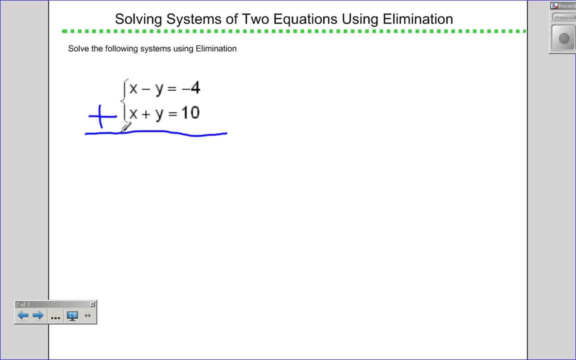 So I'm really just going to make this a giant plus sign- I call this kind of the big plus sign method- And combine our equations. So let's say x plus x is 2x Negative, y plus y is nothing is zero. 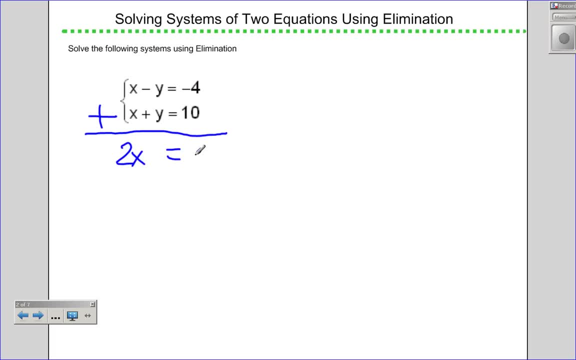 Bring down my equals Negative: 4 plus 10 is 6.. And now I have just one variable, that x. I can solve for x, So x equals 3.. Remember, the solution to any system is the point, So I'm always looking for that point. x, comma y. 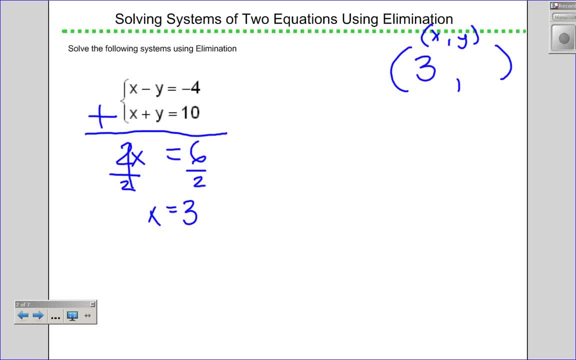 So I've just gotten my x value of 3.. Now, I can't necessarily do this. I can't necessarily do it for the x value as well. I could go back and do it again, But I just basically need to pick one of these now and plug in my x. 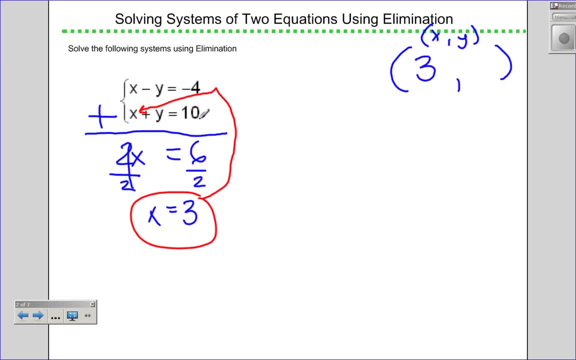 So I'm going to choose the second one because it's plus and I have a positive And I could have chosen the first one. it doesn't matter as long as I pick one equation to find out the y value. So I know x plus y is 10.. 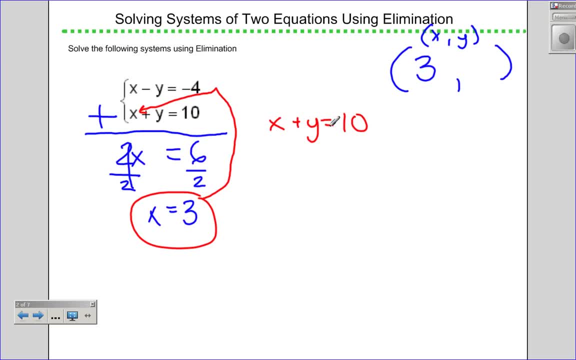 I always like working with addition and positive numbers, so that's the only reason I chose this one. I know x is 3, from right here. So 3 plus y is 10,, so y equals 7.. So I have my y value now, so my answer is 3 comma 7.. 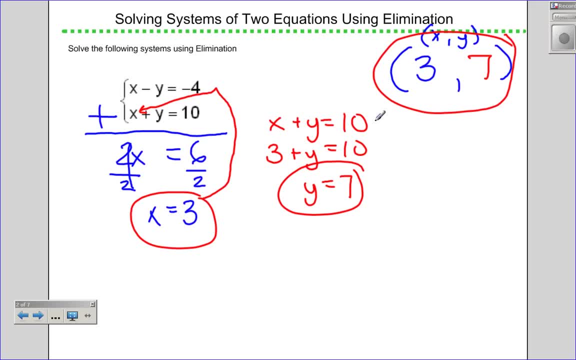 Remember, the solution to any system is the point where the two lines intersect. So I have 3 comma 7. So I was able to eliminate one of the variables by combining. This is also sometimes referred to as the combination method. I'm combining the two equations to get rid of one of the variables. 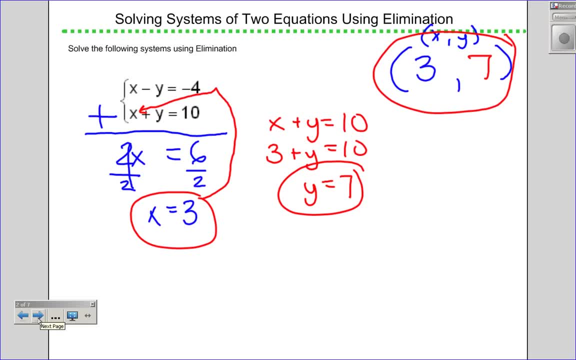 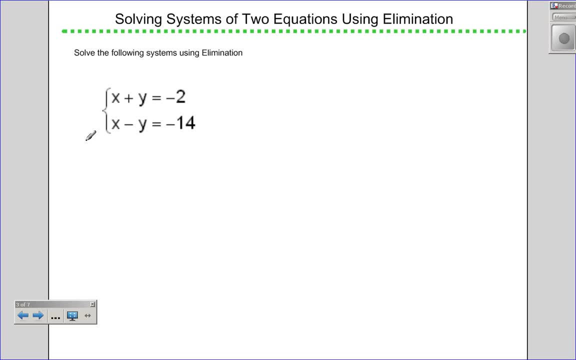 I chose the y values because they were opposites. in this case I'm always looking for those that have the same kind of coefficient and our opposites. So in an example two here I'm going to do a very similar thing. Just make my big plus sign. I notice I have opposites in the y's, So I can. 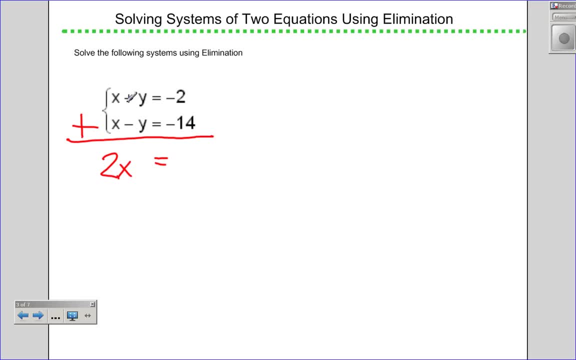 combine: my x plus x is 2x, The y's cancel or they eliminate each other. And negative 2 plus negative 14 is negative 16.. So x equals negative 8.. I got to set up my answer over here, x comma. 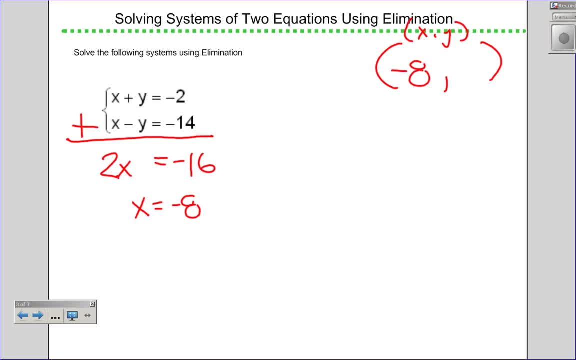 y is going to be my answer. So I have that x value of negative 8.. Now I'm looking for my y value. I'm just going to choose the first one, because it's plus over here And it's a negative 2,. 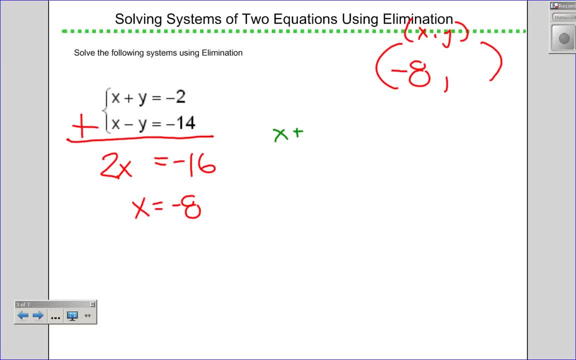 which is a little bit friendlier than negative 8.. So I have x plus 2 or x plus y- excuse me, equals negative 2.. So let me just kind of start over here. So x plus y equals negative 2.. 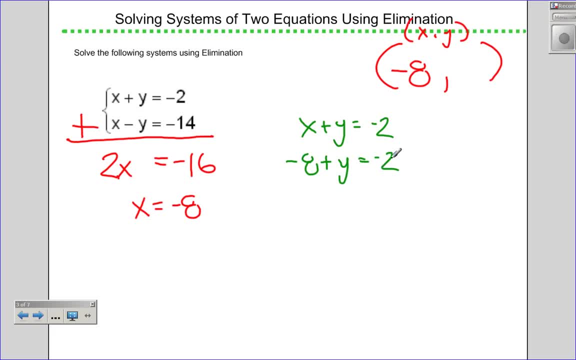 I negative 8 plus y is negative 2, add 8 to both sides, so y equals 6.. That is my point of intersection there of my two equations. My answer, my solution, is negative 8 comma 6.. Let's look at another one here, another system of. 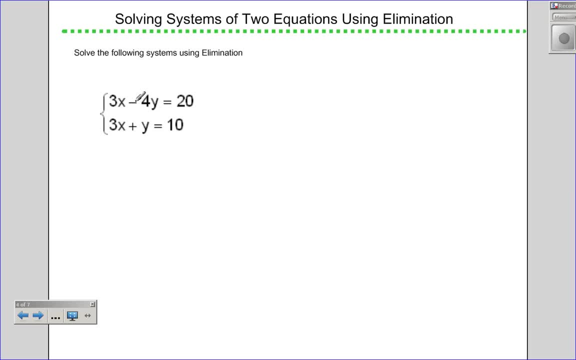 equations that we'll solve using elimination. So I'm going to look and my y's don't cancel in this one and I have a positive 3 and a negative 3.. So I can't necessarily use the big plus sign, but what I can use is the big minus sign. So 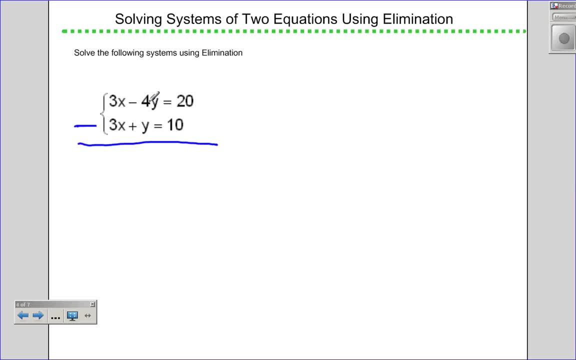 I have 3x minus 3x, 0 x's Negative, 4 minus 1 would be a negative 5y. 20 minus 10 is 10.. So y equals a negative. 2.. My answer up here: x comma y. I always want to make sure I have. 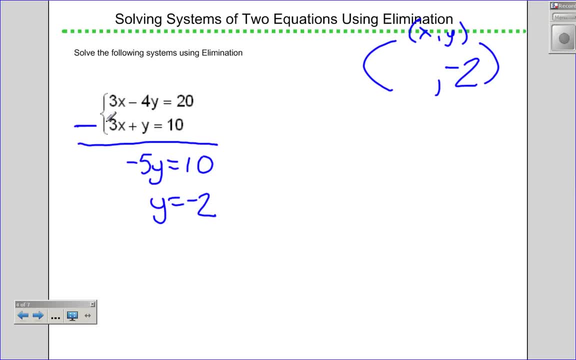 that answer. So I have negative 2 for my y value And now I need to pick which one of these I want to work with. I'm going to work with just the second one, just the second one. So I'm going to work with the second one. So I'm going to work with. 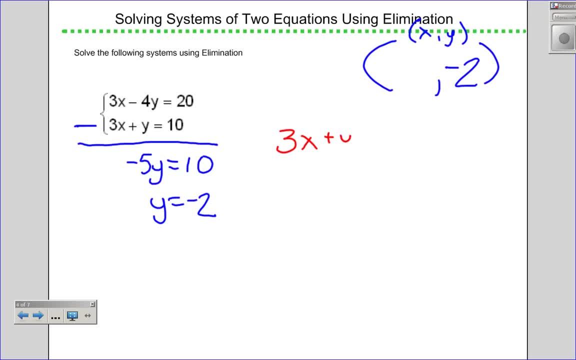 just because it's a little more friendly looking to me. And once again, it doesn't matter, You can choose whichever one you'd like to choose. So I have 3x plus negative 2 equals 10.. So 3x minus 2 equals 10.. Add the 2 to both sides: 3x equals 12.. So x. 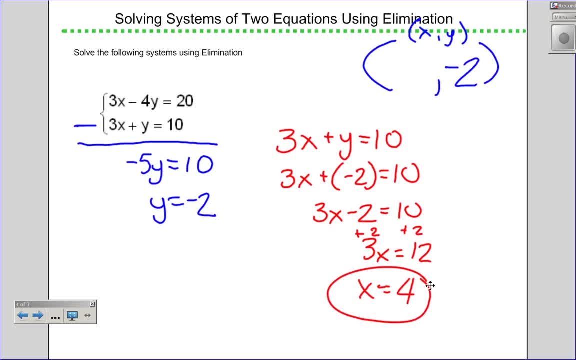 equals 4.. And that becomes just my second point up here of excuse me. my second point up here of excuse me, 4 comma negative 2. And if I plug it in I would get 3 times 4 is 12 minus a negative 8.. And I can add that, So 12 plus 8 is 20.. That verifies. 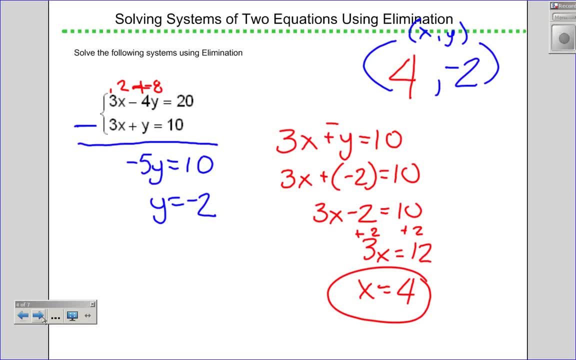 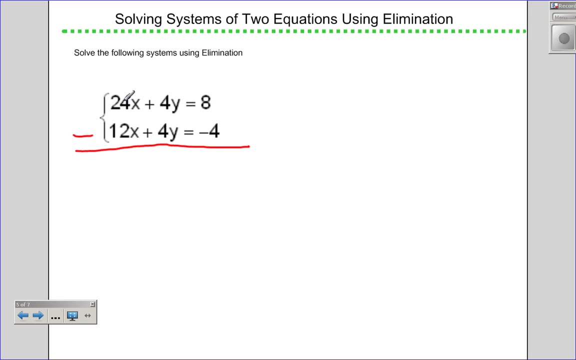 12 minus 2 is 10.. It checks out in both equations, And let's look at our next one here. So once again, I don't have opposites that I'm starting with, But I do have the same coefficient of the 4y, So I can subtract them. 24x minus 12x is 12x. 4y minus 4y cancels. 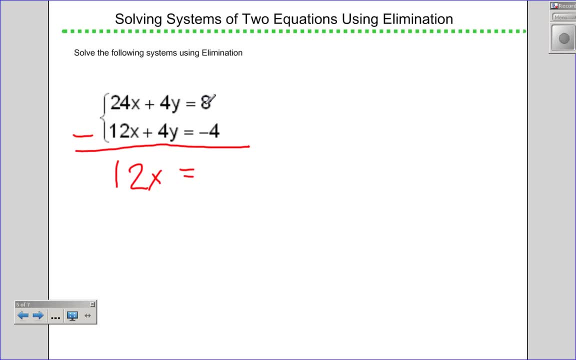 They eliminate, And 8, this is- you have to be careful here- 8 minus negative, 4 means minus a negative 4.. I'm going to add those together, So that's 12.. So x equals 1.. So I have my answer- x and y. So x is 1.. I'm looking for my y value now. 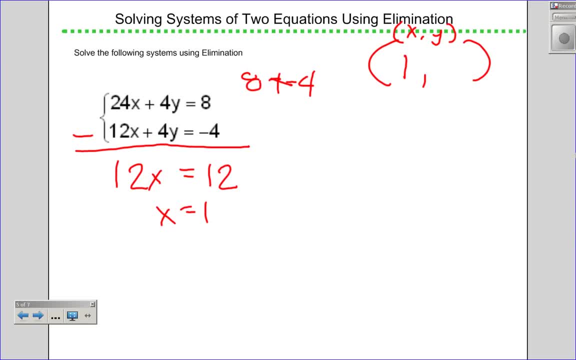 I'm going to just pick the first one, because it's all positives And I like working with those positive numbers, as you know by now. So I have 24x plus 4y equals 8.. 24 times 1 plus 4y. 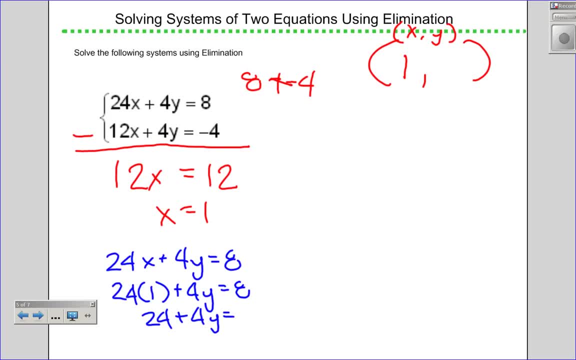 equals 8.. 24 plus 4y equals 8.. 24 times 1 plus 4y equals 8.. 24 times 1 plus 4y equals 8.. 28 times 1 plus 4y equals 8.. 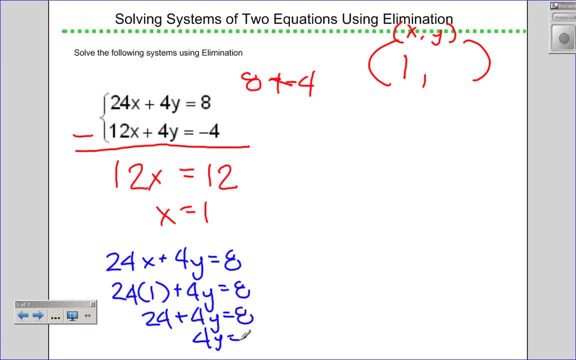 28 times 1 plus 4y equals. having 4y equals subtracted 24 from both sides gives me a negative 16. So I am just going to move over a little bit. So 4y equals negative 16. So y equals. 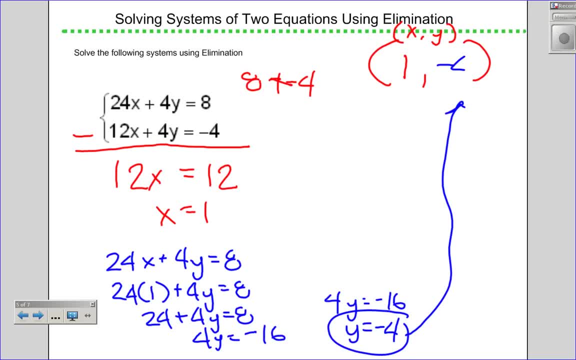 minus 4.. So I can take that, plug that in up here And there is my solution to this system of equations using elimination. Now could I re-written these in ends and slope intercept form and graph them? graph them: Yes. Could I have rewritten it for one of the variables and did substitution? Yes. 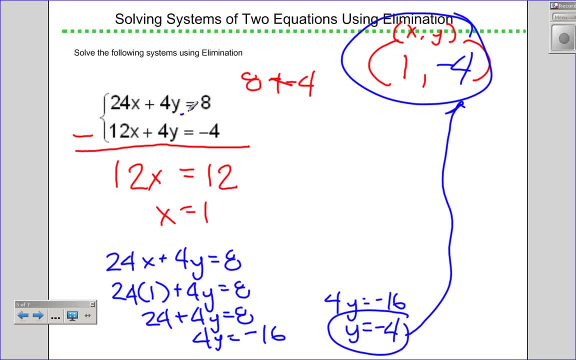 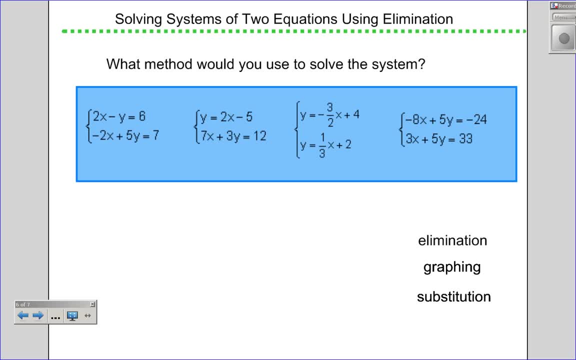 Would have been very laborious, intensive in order to do that, but I could have done it that way as well. So let's take a look here. So what method would we use to solve these? So if I'm looking at the like this equation here, this first one, 2x minus y is 6 and negative 2x plus 5y is 7.. 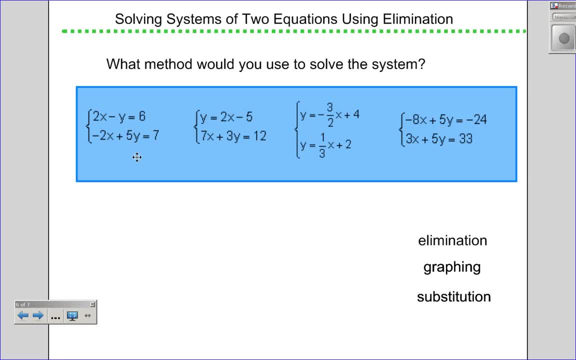 Do I want to graph these? Do I want to use elimination or use substitution? So I noticed that they're not written in slope intercept form, so I probably don't want to graph them. I don't have one variable written for the other variable, but I do notice that I have the same. 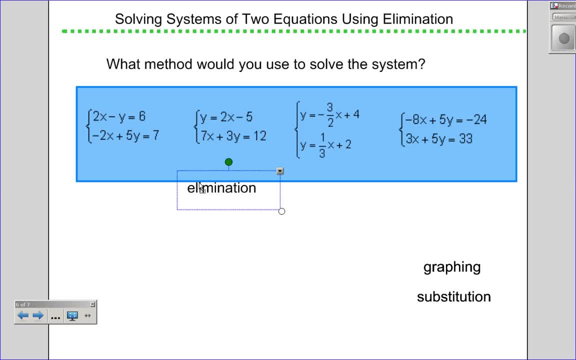 opposite coefficients here in the x's, so I can use the elimination method. I have: y equals 2x minus 5 and 7x plus 3y equals 12.. Well, I have the first one. It's written so I can graph it pretty nicely, but the second one's not. But the first. 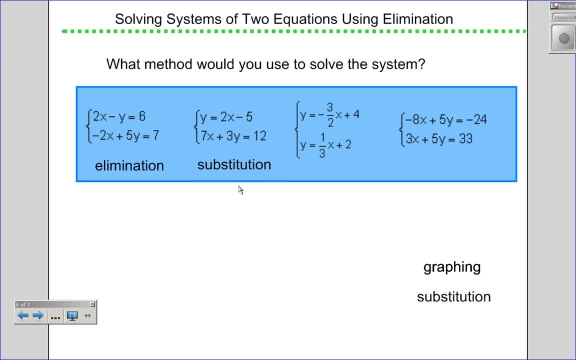 one's also written for one of the variables, so maybe I want to substitute that. Let's take a look here at this third one: y equals negative 3 halves x plus 4, and y equals 1 third x plus 2.. Well, they're both written for a variable, so maybe I could substitute. 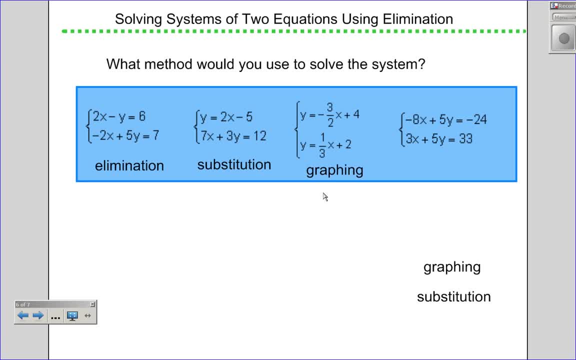 but they're also written pretty nicely in slope intercept form so I could really graph those pretty easily too. So maybe I would do that: Negative 8x plus 5y equals negative 24.. 3x plus 5y equals 33.. Well, they're not written in slope intercept form like this one, so I don't want to graph. 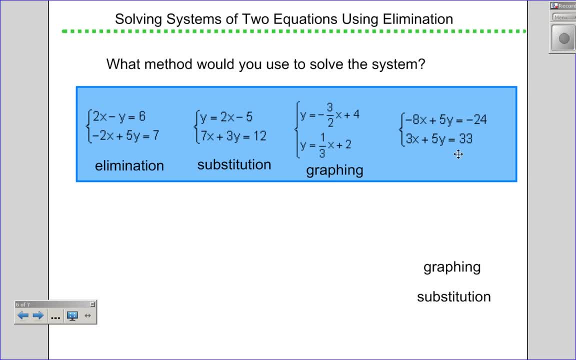 them. They're not written for one of the variables, so I don't want to use substitution necessarily, But I do notice that 5y's are the same, so maybe I could use the elimination method as well for this one. So do that for this case here. So I would use elimination for both the first one and